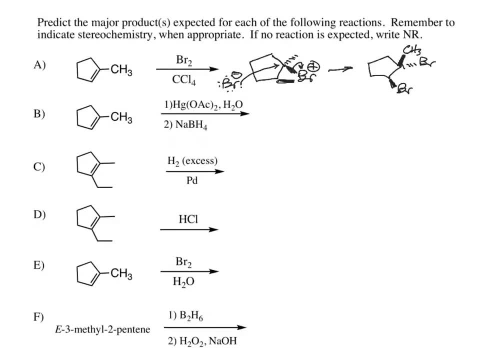 that the methyl group gets pushed out as a wedge. So this is one product and of course it doesn't matter which bromine is going to be pushed out as a wedge. So this is one product and of course it doesn't matter which bromine is the wedge and which bromine is the dash. So we always want to. 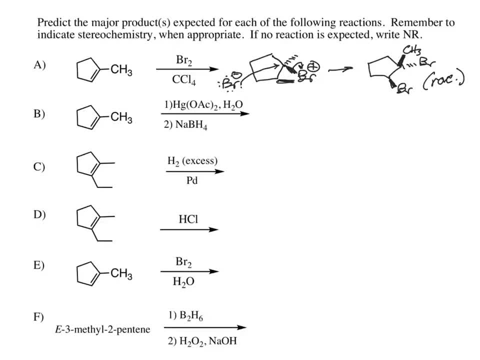 indicate that this is racemic, because we just formed a chiral product from an achiral starting material, So we can indicate that it's racemic. or we could say plus enantiomer, or something like that. Okay, our next example is described as an oxymercuration. This first step is called an. 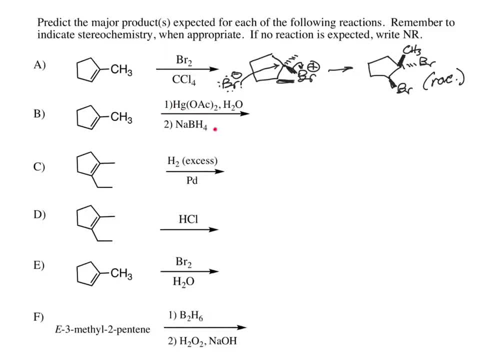 oxymercuration step. The second step is called the demercuration or a reduction step, and the process, that two-step procedure, is going to break the pi bond and add two groups across the pi bond. It's going to be a hydration, It's going to 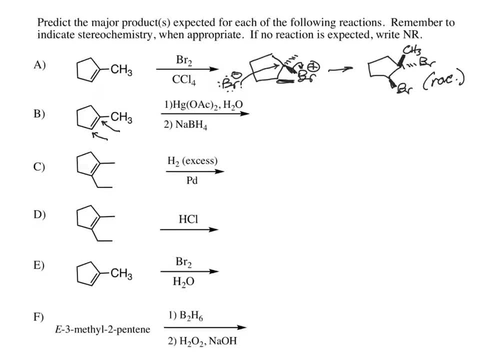 add an H and an OH, and this reaction proceeds with Markovnikov addition, which means the hydrogen goes to the carbon with more hydrogens and the OH goes to the more substituted carbon. Now this is going to give us mixed stereochemistry, but in fact, because we're not creating any new chiral centers, 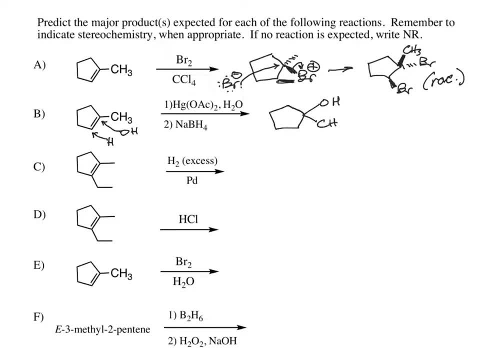 in this example, since we're not creating any new chiral centers. there's actually no chemistry to show. this is a symmetrical molecule, It has no chiral centers, and so if you want to draw the hydrogen, you could draw the hydrogen, that's fine, or you could leave it off, because it's just. 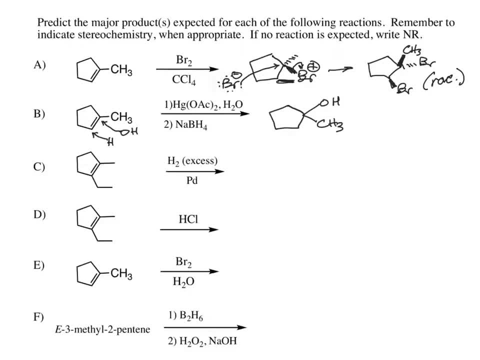 a line drawing, So we'll get this tertiary alcohol as our final product. In the next case we have catalytic hydrogenation, So I have H2.. Again, we could always assume everything's in excess, but we've pointed it out here, and palladium is going to be the metal catalyst that's needed. Okay so, 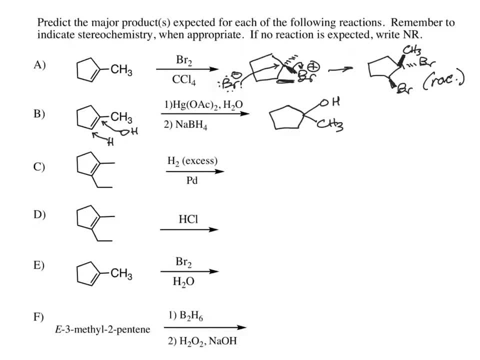 we're going to break the pi bond and we're going to add a hydrogen to it. So we're going to add a hydrogen and a hydrogen across the pi bond and this is going to occur with with a particular stereochemistry, We observe sin addition of the two hydrogens. That means they're going to add to. 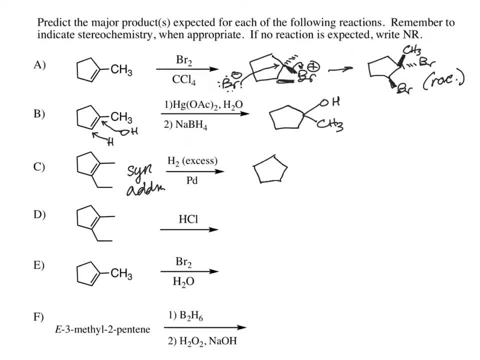 the same face. So in the product we need to show both those hydrogens as coming from the same face. So in other words, they can both be drawn as wedges, or they could both be drawn as dashes, but hydrogens come in as the as wedges, then that means it's going to push the alkyl groups that are initially there. 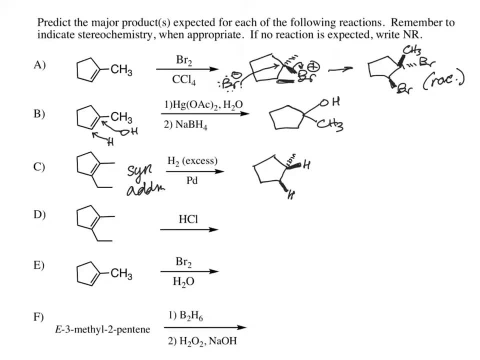 back to be dashes. So I have a methyl on this top carbon and I have an ethyl on this bottom carbon. Okay, and again, plus enantiomer or racemic to indicate that the hydrogens can also come from the bottom face. This is a chiral. 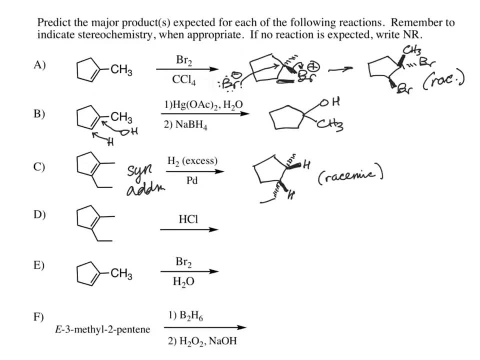 molecule, so we would have to indicate that it's an enantiomer- is also formed. Okay, in our next example we're adding HCl across the pi bond, So we're going to add HCl across the pi bond. Normally we would expect to do this with Markovnikov addition, where we want the 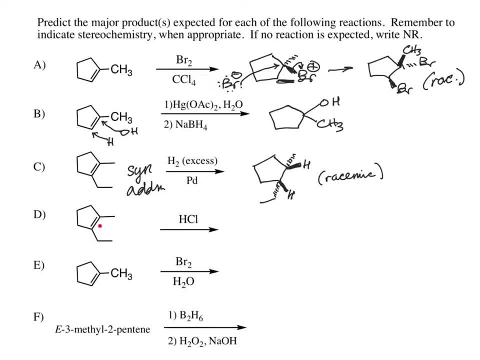 hydrogen to go to the carbon with more hydrogens. but in this case neither the carbons have hydrogens. and remember the rationale behind Markovnikov's rule is: you want to get the most stable carbocation possible, but if I protonate at either position I'm going to get a tertiary carbocation. So let's. 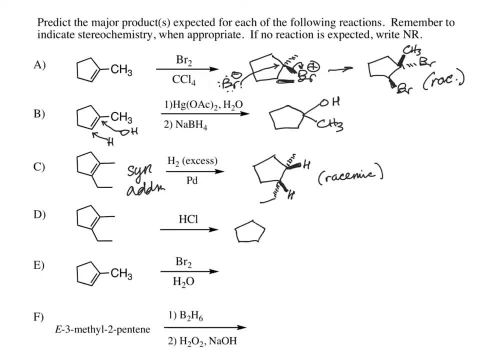 take a quick look at that, My two possible carbocations. I can either protonate at the top carbon to give this carbocation, or I can either protonate at the top carbon to give this carbocation, Or I could protonate at the bottom carbon to give this carbocation and notice that they're both tertiary. 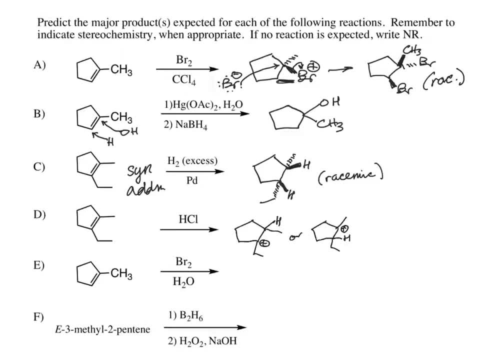 so they're equally stable. and if I have two equally stable carbocations, I expect them both to be formed, and so they're both going to lead to our final, our major product, significant projects. So that's the first step in the mechanism. So protonation: we can show that mechanism here, So we protonate. 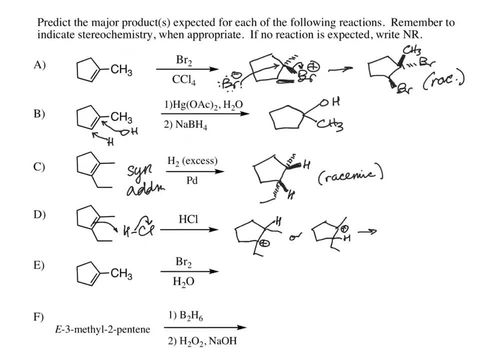 the pi bond with two arrows, and to do that we're going to protonate at the bottom carbon to give proton transfer. It happens with either regiochemistry, and so then, when the chloride that was formed in our first step comes back as a nucleophile, I can add to either of these. 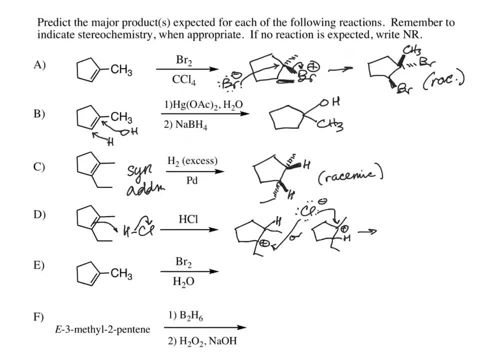 carbocation ions and we're going to get a mixture of regiochemistries. The other question here is: what about the stereochemistry? This is not a stereospecific reaction, because the hydrogen is added in one step and the chloride is added in the second step, So in other words, it doesn't. 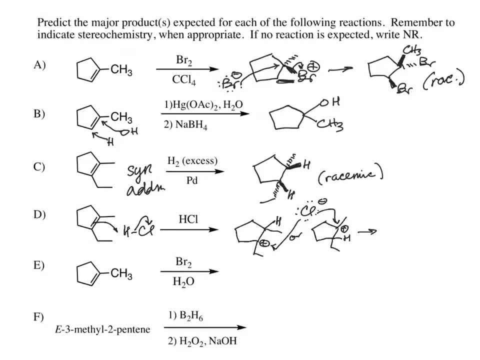 happen with only syn addition, where they come from the same face, or only anti-addition, where they come from opposite sides. So we're going to get a mixture of the stereochemistry. and the other question here is: what about the stereochemistry? This is not a stereochemistry, So we're going to get a. 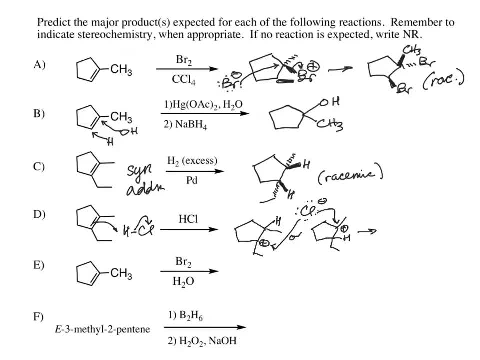 total mixture of stereochemistry. So in that case what we should do is we should. we'll just draw them as flat as everything is flat lines. So if the first product would have a chlorine on the bottom carbon and the second product would have a chlorine on the top carbon, It doesn't matter. 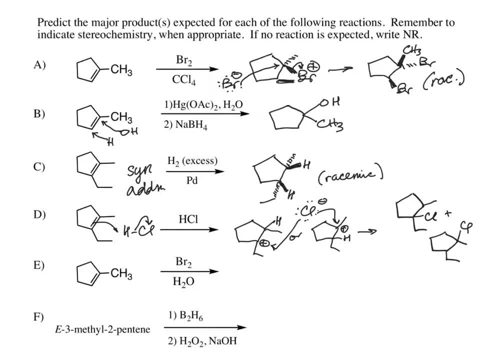 where you draw them. there's no stereochemistry to show. So in other words, this: this would have the if we've just focused on the two alkyl groups. the two alkyl groups can be cis to each other, they could be trans to each other, and then, of course, each of those would have both enantiomers. 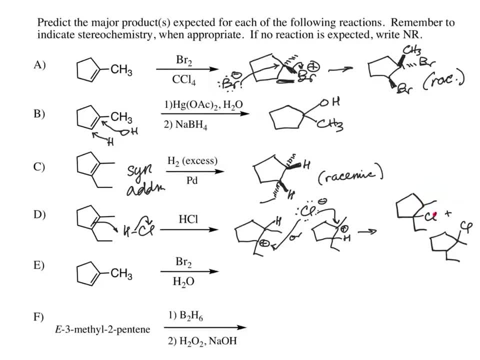 So there's four different ways it says because it says two chiral centers. there's four different ways you could draw this compound. four different stereoisomers, four different ways you could draw this compound. So in fact there are eight products. there are eight products, possible products you can. 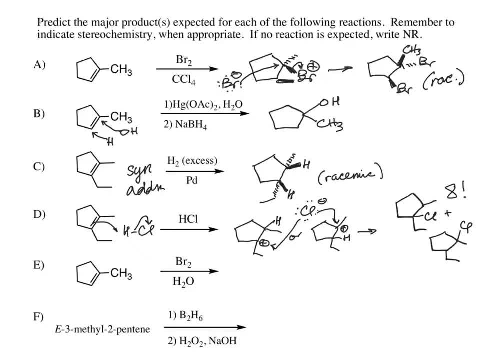 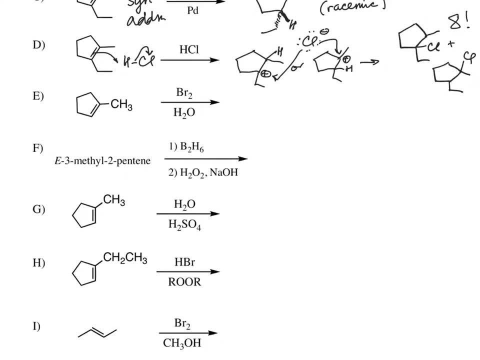 draw. So that's why we're just going to draw them as straight lines, because there's no significant, um significant stereochemistry to indicate. Okay, let's take a look at our next reaction. here we have bromine again. Okay, anytime we have bromine. 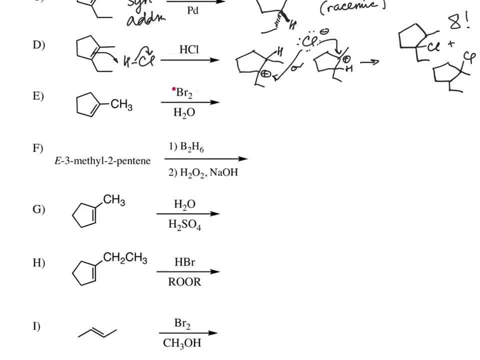 reacting with an alkene. the very first thing that's going to happen is we're going to form a bramonium ion. Okay, but now we have a solvent that is not like carbon tetrachloride. that is not going to be involved. our solvent now is nucleophilic, and that's going to be what attacks. 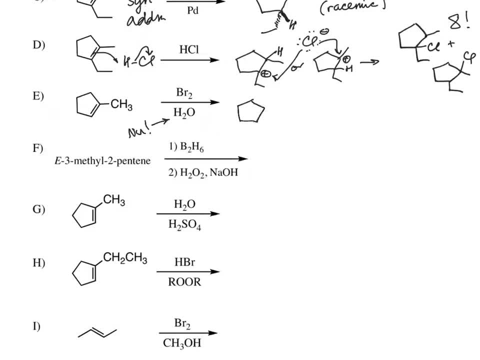 bramonium ion. a look at what the bromonium ion looks like. I'm going to skip our stereochemistry here just for a second. sorry, I'll add it in. So if we imagine the bromonium ion coming in as a wedge, we are. 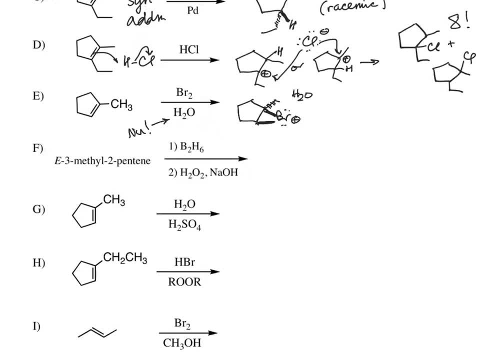 now going to have the water come in as our nucleophile, and the water has a decision to make on which carbon to attack. And what's observed is, when I compare these two carbons, okay, we see that this carbon, because it is tertiary, it's going to be. 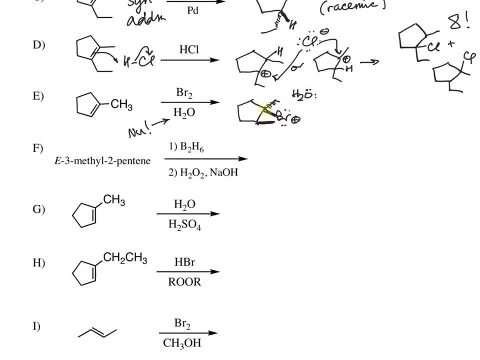 more electrophilic because the partial positive is stronger there. it's better there because it is a tertiary partial positive, and so that's where the water is going to attack. So, remember, that's going to be a reflection in terms of what we're seeing. So we're going to have a 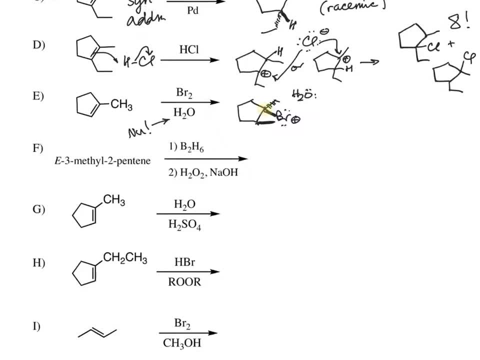 unusual for backside attack. for sn2, we usually don't want to go to the more sterically hindered carbon, but because this has some sm1 character, because- oops, let's go back to my regular marker, sorry, because this has some sm1 character due to that positive charge, it's going to actually be. 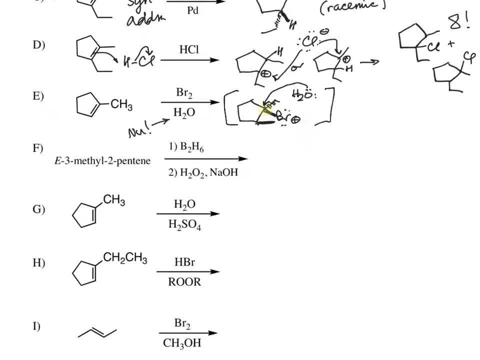 attracted to the more, uh, substituted carbon. so it's going to attack at the more substituted carbon. this is backside attack. so if i attack this carbon, that's the carbon bromine bond that i break and again we're going to see that backside attack. the sn2, we're going to see, um, the anti-addition. 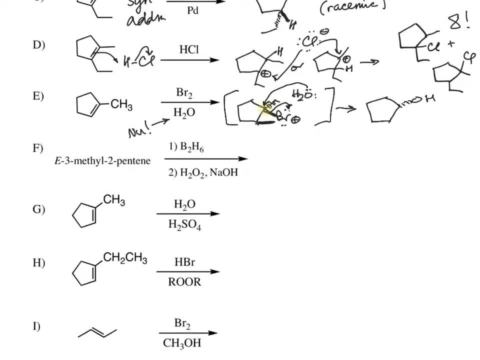 so when we're done here, the oh is going to be a dash and the br is going to be a wedge, so we get anti-addition, just like if we had br2, and the oh and the br end up trans to each other. so what happens to this methyl group that we 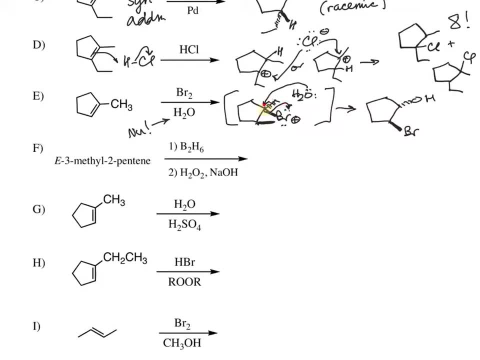 had here. this methyl group was a dash, but we get inversion at that site, so, um, the oh ends up being a dash and the methyl group ends up being a wedge, so we could draw that right here. okay, once again we've drawn a chiral product, so we can't just have this one product, form it also. 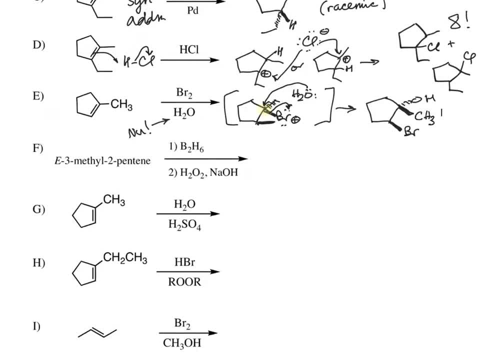 has to be uh, plus it's an antimer, so maybe we could write that: so plus an antier. whoops, that's not how you spell an antimer, that doesn't look good. plus, plus in the antimer. there we go. or you could say racemic, or you could uh have some other indication. 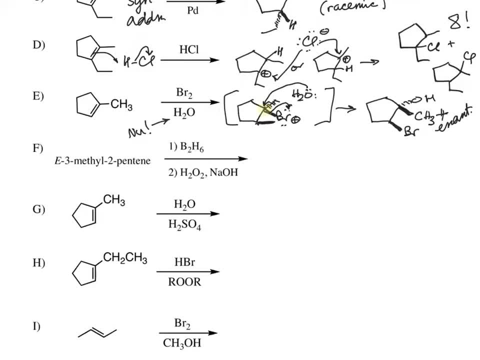 that it's going to be a racemic mixture. so in other words, when the first bromine attack, when bromine first attacks, this bromonium ion could have come from. the, could have formed from the bottom face. so the bromines, two bromine bonds, would be dashes and then the water would have. 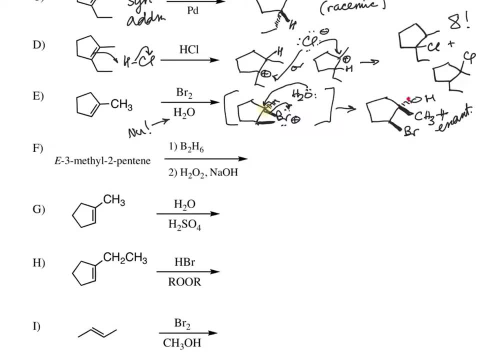 to attack from in front of the page, and so the oh would end up as uh, the wedge. so ultimately, we want to make sure that we get these two groups anti to each other. um, because of the br and the back side attack mechanism. okay, our next example is a hydroboration oxidation: two steps: hydroboration. 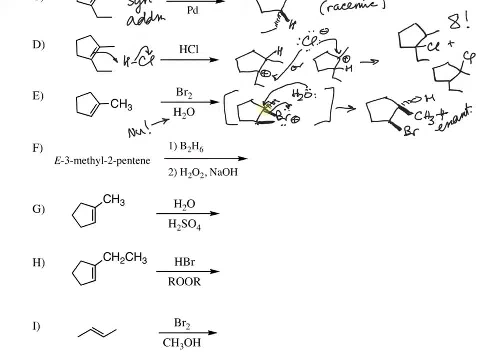 oxidation. okay, this is going to give uh anti addition, and the groups that are going to be added are the components of water. we're going to add an h and an. oh, we're going to add a hydrogen and a hydroxyl group. so first we have to figure out. 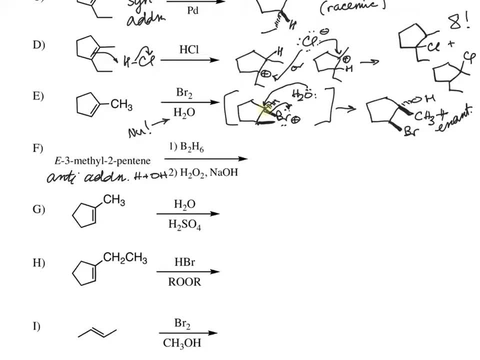 our structure looks like: we have uh, e, three methyl, two pentene, so let's draw two pentene, so there's pentene, and we add a double bond here, and so at carbon three we have, um, a methyl group, one, two, three. this is where a methyl group is, and 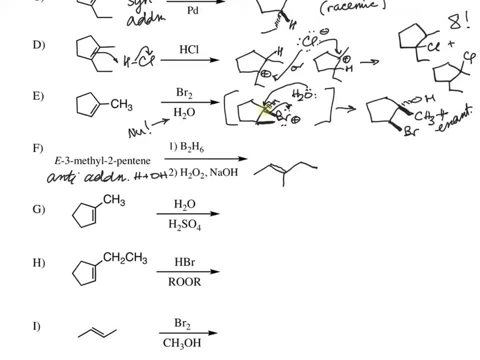 um, let's check to see if i just accidentally, in drawing my first drawing, came up with the e stereo chemistry. okay and uh, in order to figure out if this is e, we look on each carbon, we look at the two groups on each carbon, on the two. the two groups on this carbon are just a. 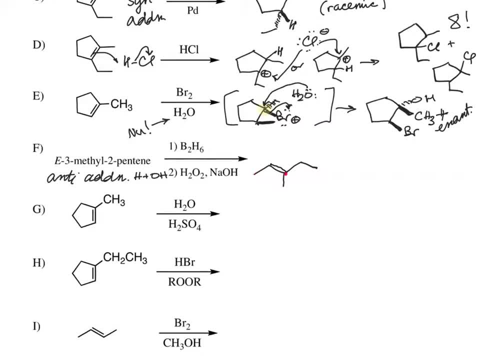 hydrogen and this methyl. so the methyl is the higher priority. on the second carbon, we have a methyl and an ethyl. the ethyl is higher priority and because the um highest priority groups are on opposite sides, they're trans to each other. this is in fact this, the e stereo chemistry. so i kind 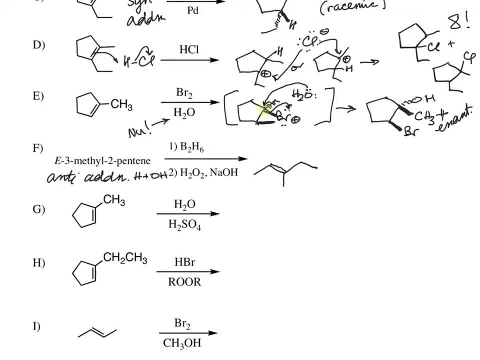 of lucked out there, when i, uh, when i drew it as a line drawing, if this, uh, if i maybe started with the z, okay, maybe if i or i didn't draw it right the first time, what i would have to do is simply swap two of these groups right, or either put the methyl 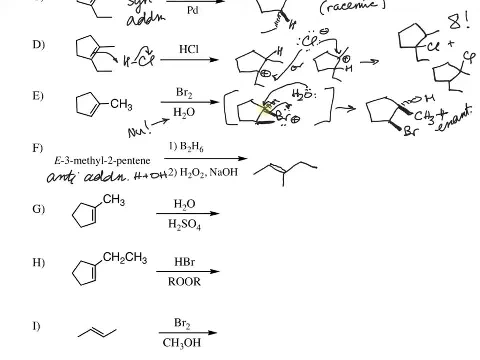 group up here instead of down here, and that would be the z stereo chemistry. okay, but we were supposed to start with e, so that's good. so what are we going to do? we're going to add two groups across the pi bond, we're going to add an h and an oh, and we're going to do it with anti-mercombat. 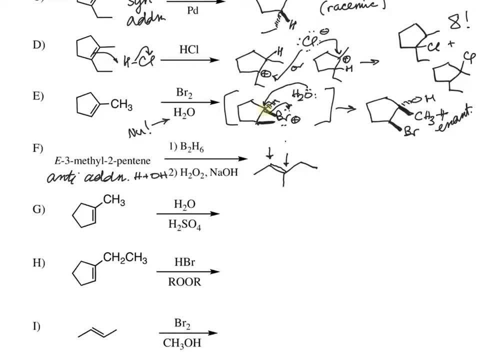 the hydrogen goes to the carbon with less hydrogens. so the hydrogen is going to go on the more substituted carbon, the oh is going to go on the less substituted carbon and we also um get, uh, i'm. i'm looking at my text here and i realized that i was saying anti-markovnikov. 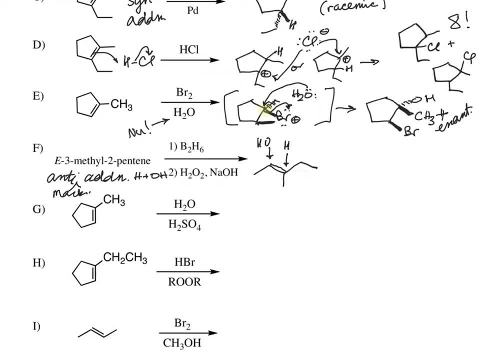 addition, but i didn't write that, so this is anti-markovnikov describes the regiochemistry, but the stereochemistry is defined when the hydrogen and the boron add in the first step and that is syn addition. syn describes the regio, the stereochemistry they add from the same face. 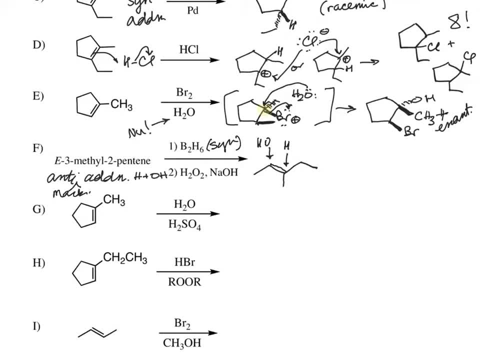 so when we draw our product, when we draw our product, we want to add the h and the oh from the same face. so let's make them both wedges. for example, the wedge bond is up here for a zigzag up, it's down here for a zigzag down. 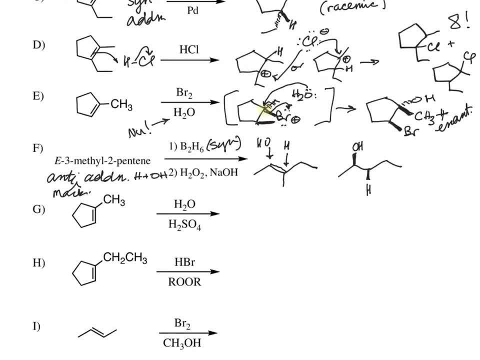 so that would be syn addition, both from the top face. and then what's that going to do to our existing methyl group? if my hydrogen came in from the top face, that's going to push the methyl group back to be a dash. so that would be one way to draw it. the other way to 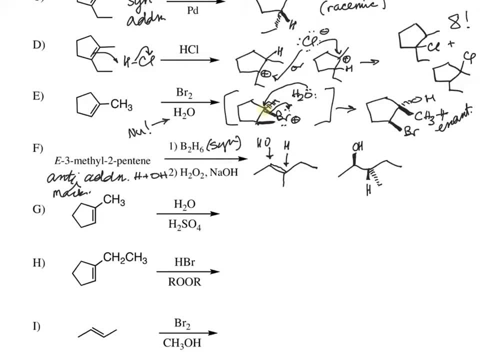 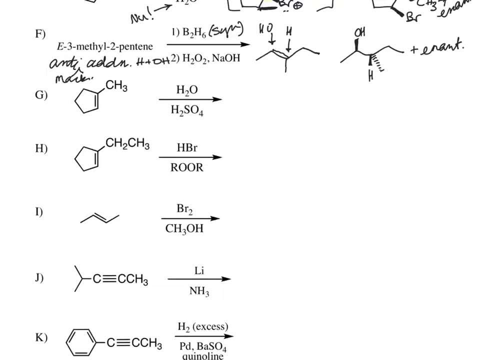 to draw, it would be have the h and the oh be dashes instead. so again: plus enantiomer, plus enantiomer- very good. how about our next step? the next example is just water and acid. so this is the same as saying h3o plus dilute sulfuric acid, and that would be hydration conditions. so i'm going to break the pi bond. 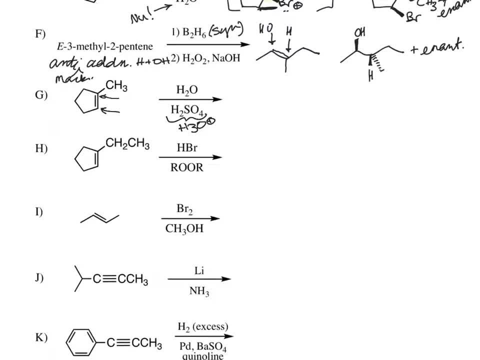 i'm going to add an h and an oh, and this is uh. starts with protonation of the pi bond, and so we're going to do it in such a way to get the most stable carbocation possible. so we're going to follow markovnikov's rule. the hydrogen is going to go to the more substituted. 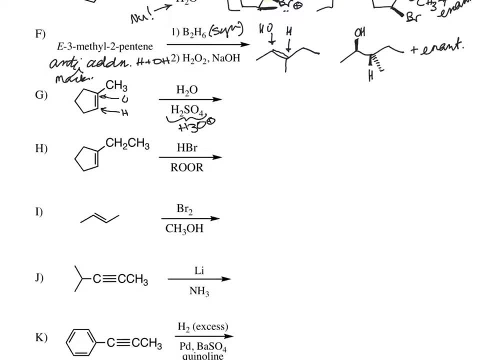 the one with more hydrogens, so that the positive charge goes to the carbon. with more carbons we get a tertiary carbocation and um and that's what it would attack. so again, just we can point out why this regiochemistry is formed. we get the tertiary carbocation is more stable. 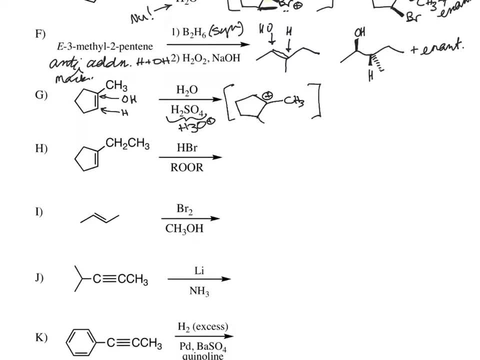 and so that's why we added the hydrogen, and so we're going to do it in such a way to get the hydrogen to the carbon that already had more hydrogens. and so water is going to be my nucleophile and it's going to attack the carbocation, and then we're going to have to deprotonate the water to. 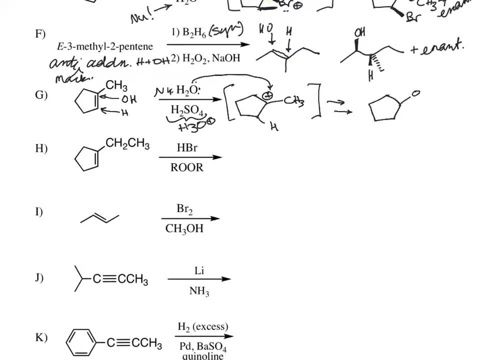 make it neutral and we're going to get an oh, a tertiary alcohol, and now again, this is another example where there is no fixed stereochemistry, that's of a relationship between the h and the oh that we're adding, but also in this case we have a symmetrical molecule. we don't have any. 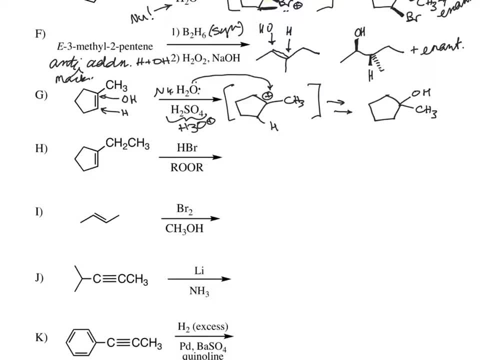 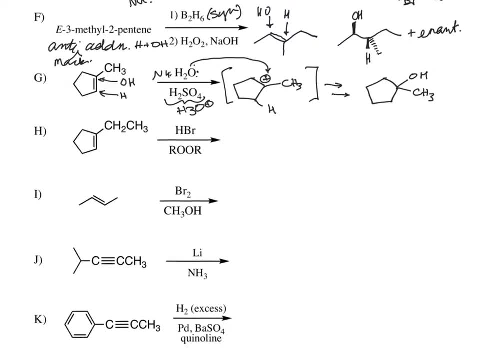 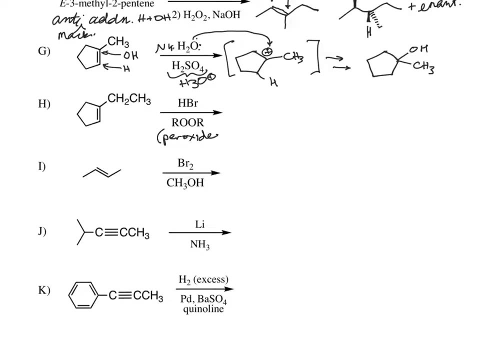 chiral centers, and so this is just the tertiary. alcohol is what we've formed here. okay, our next example is addition of hbr. but we have a special addition here: we've added peroxides, so having that oo bond is described as a peroxide and that gives a radical mechanism. 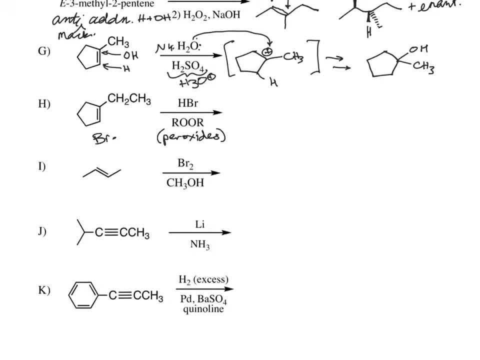 the radical mechanism is going to cause a bromine atom to add to the pi bond to give the more stable radical intermediate, which is a tertiary radical intermediate. remember, radicals have the same relative stability as carbocations, so more carbon groups would be better. okay, and because that is my intermediate, then when the it abstracts a 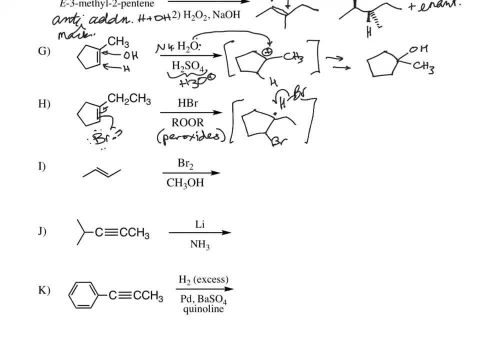 hydrogen atom from hbr. we do a, an atom abstraction. the final product is going to be um addition of hbr. but when we look at that regiochemistry we see we would describe it as anti-markovnikov- anti-markovnikov regiochemistry because the hydrogen went to the more substituted carbon. 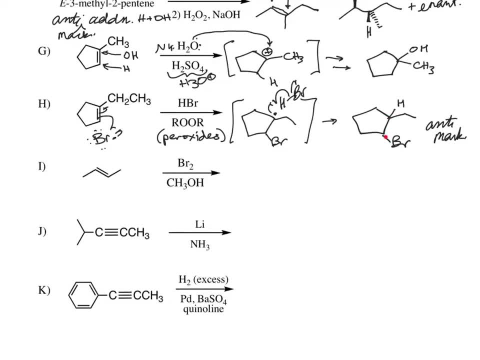 and the bromine went to the uh, the carbon, with more hydrogens. so this is the, the um. we get the opposite regiochemistry and the presence of peroxides because of this radical mechanism. uh, no stereochemistry, no specific stereochemistry to show here again, because 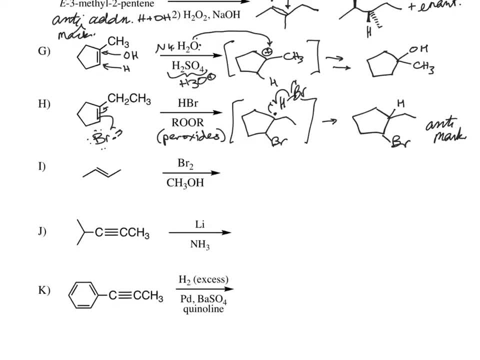 the two groups are added mustard steps. there's no um, un, Uh, no relative stereochemistry to worry about. They're not added only syne to each other, only antirere pawn in the. We're going to get all four possibilities here. we would have, uh, you know, r, r, s, s, s, r and s? r and s s long fleets. 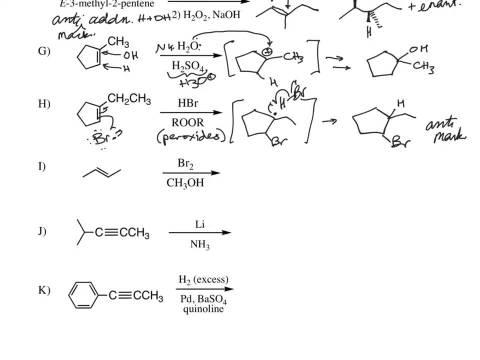 as our um four possibilities. Okay, our next example is another case where it is an Shelter- Sysad slot ring, SOS P tão sjál- where we have a formation of a bromonium ion, but we have another example of a nucleophilic solvent, a nucleophilic solvent. So that's going to be what opens up the bromonium ion And I can show. 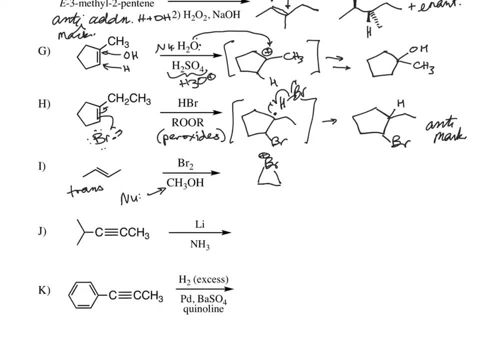 what that bromonium ion looks like. Notice we started with a trans alkene, So those two alkyl groups are still going to be trans to each other in the bromonium ion And so now when I have my methanol attack, it can attack on either side. Those would actually lead to our two. 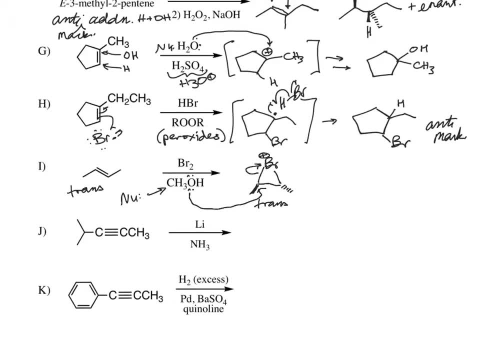 possible enantiomers, And so it's going to attack on either side And we're going to have to again deprotonate. So when methanol acts as our nucleophile, it is the methoxy group that ends up adding to the compound. So we can draw it if we keep our carbon chain fixed. 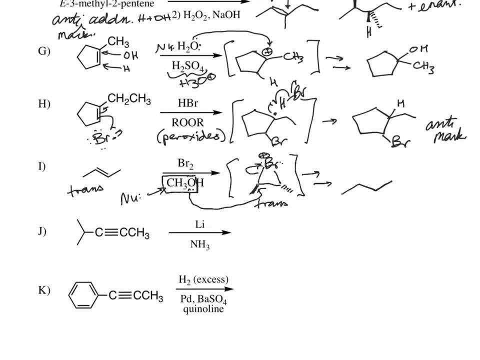 with the same stereochemistry we had in the beginning. again, we want to show that anti-addition of the two groups, the bromine and the methoxy group, because this again is backside attack. So if we draw the 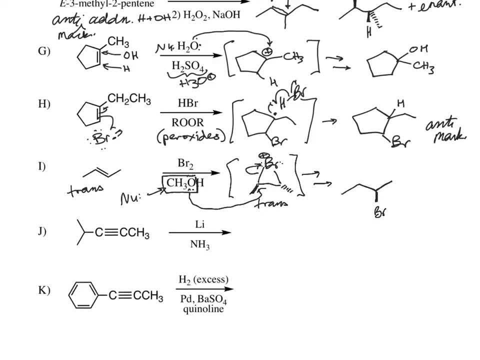 bromine as a wedge, then the methoxy group has to be a dash. The methoxy group has to be a dash. That would be one way to show it, And this is a chiromolecule, so we would want to indicate that. 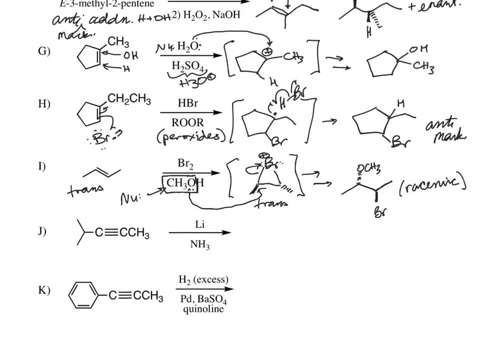 it's racemic. So again, you could either write it racemic or you could say plus enantiomer. Either way indicates that the other possibility is fine too, where the methoxy is the wedge and the bromine is the dash. Okay, and our last two examples are: 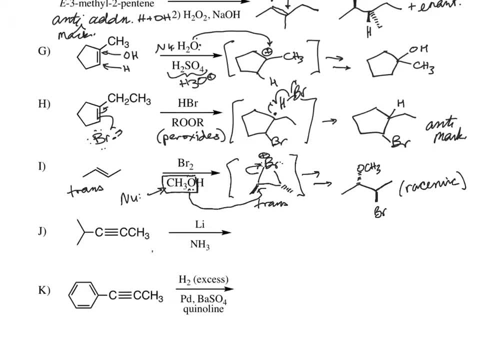 reduction reactions. Lithium and ammonia is described as the dissolving metal reduction And this involves electron transfer by the lithium. This is lithium zero, so it is lithium with a single valence electron, so very highly reactant, Very good reducing agent. It wants to donate that electron.